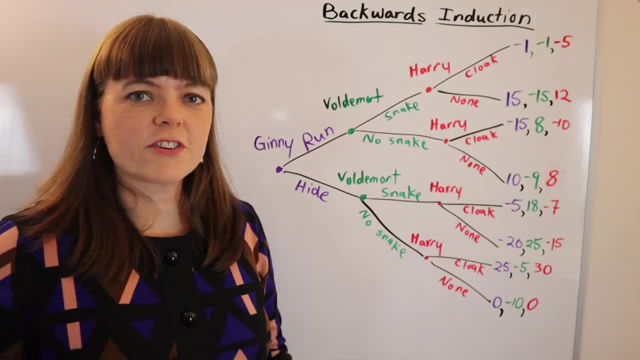 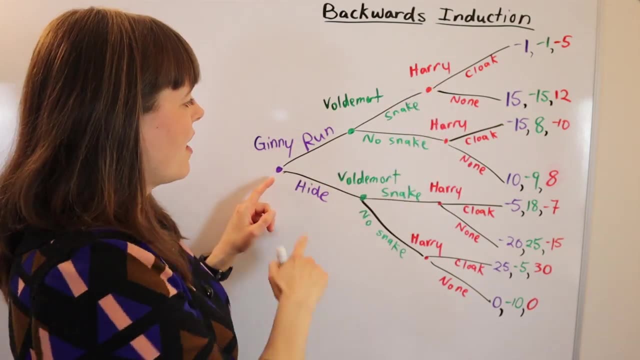 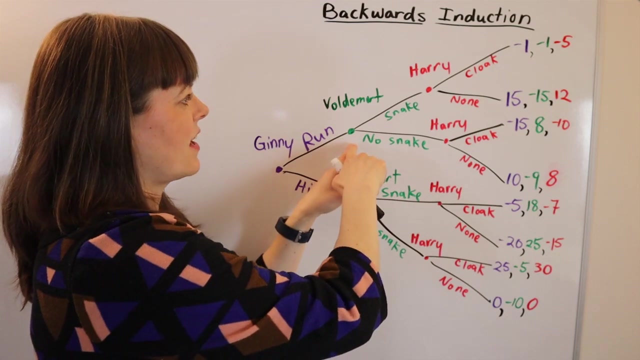 referred to as extensive form. now, first of all, i just want to set up this particular game. we have three players in this game: jenny, voldemort and harry, and jenny is deciding should i run or should i hide. voldemort is observing what she does and deciding should i bring my pet snake along with me. 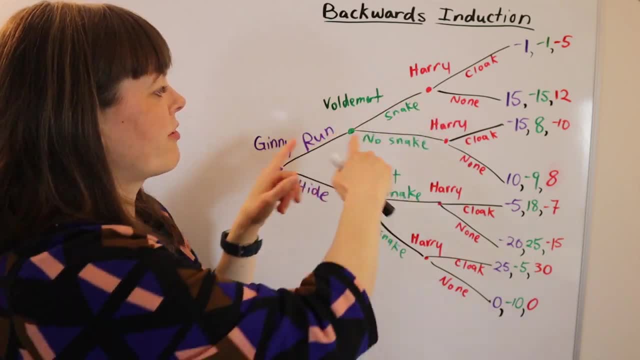 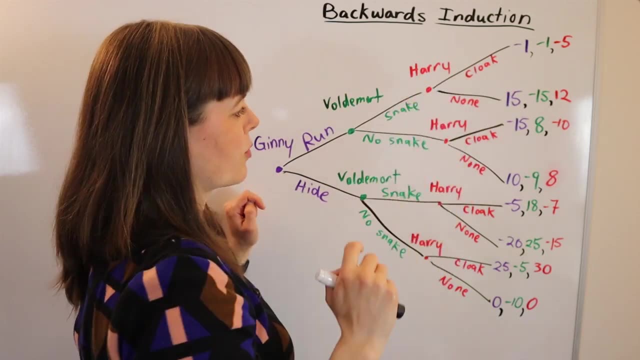 or not bring my pet snake. and then harry is observing what both of them did and then at that point he's deciding: do i bring my cloak or do i not bring my cloak? that's the game, and of course we can number our players from left to right. 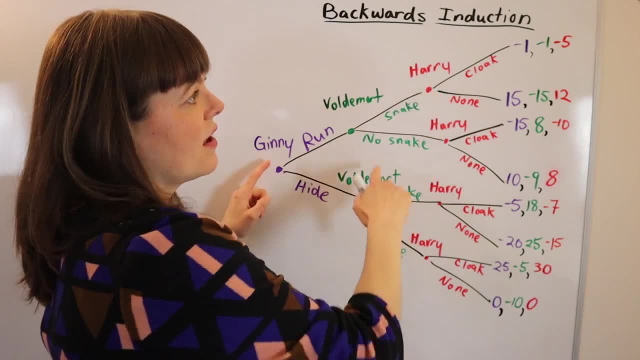 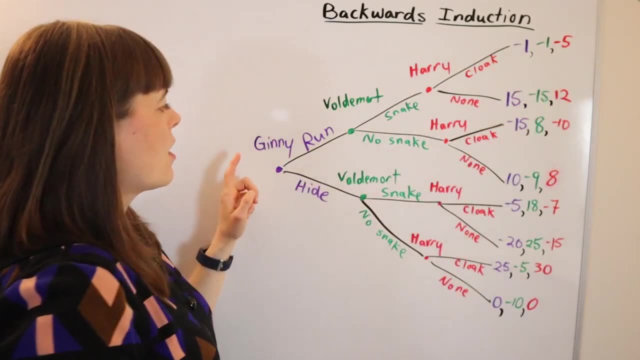 just like we always do- player one, player two, player three- and that allows us to interpret the final payoffs as player one's payoff, player two's payoff and player three's payoff, where i've color coded this, but usually you're not going to get the nice color coding. 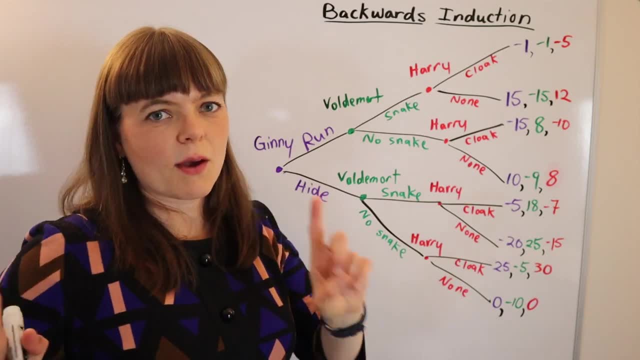 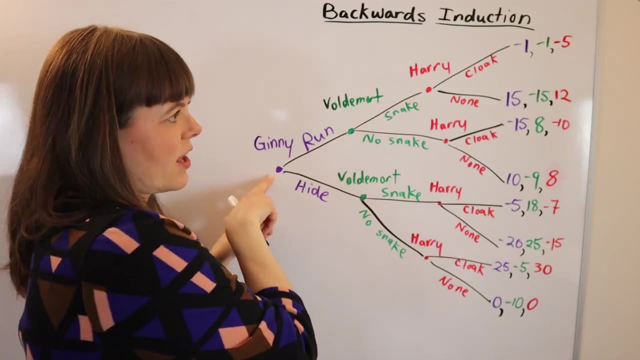 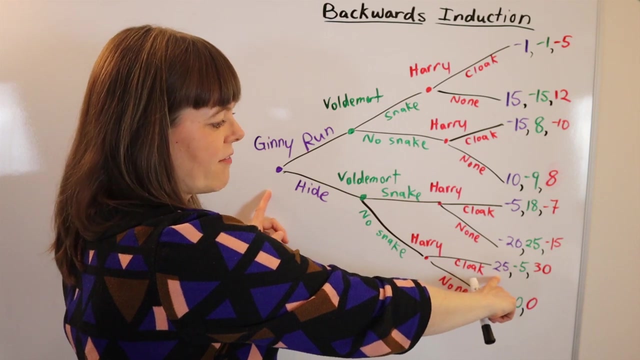 so let's get started. all right, there's actually one thing i want to do before i start, and i'm doing this just to make some points. so if jenny is looking forward into this game and she's looking at all of her payoffs, she's going to see this 25 payoff down here and say, oh, i would love to get to. 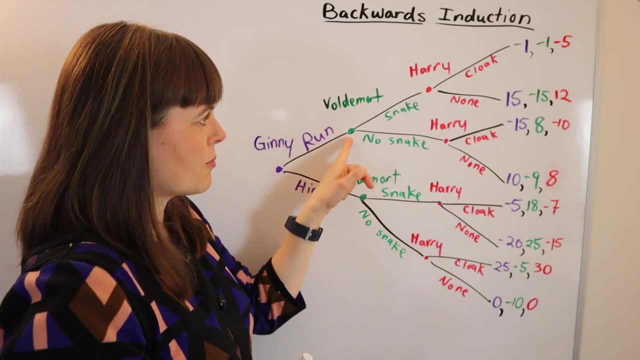 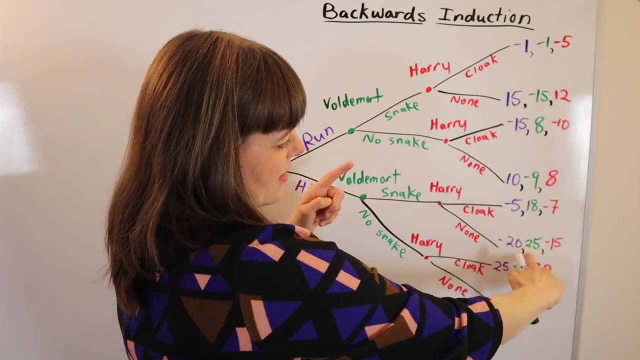 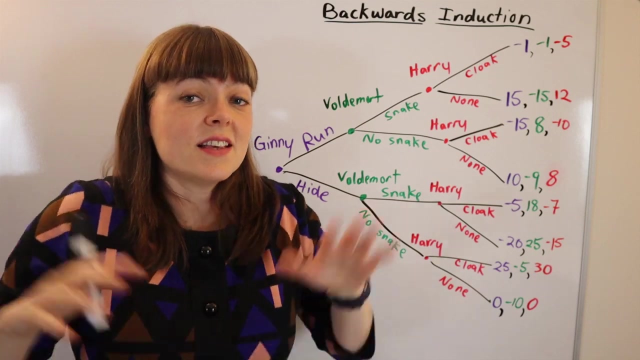 that 25 payoff and same thing. voldemort is going to look um through this and he's going to say, looking at my payoffs, i really want to get this 25 payoff, and harry, of course, will do the same thing. now, the point i'm making about this is that these players actually have no control over getting to. 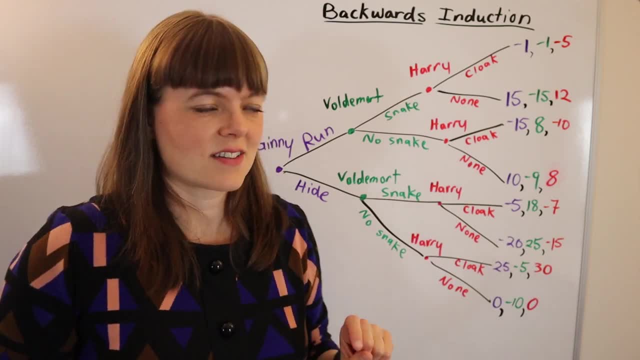 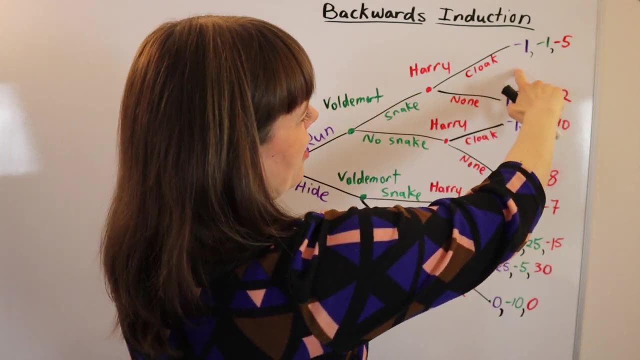 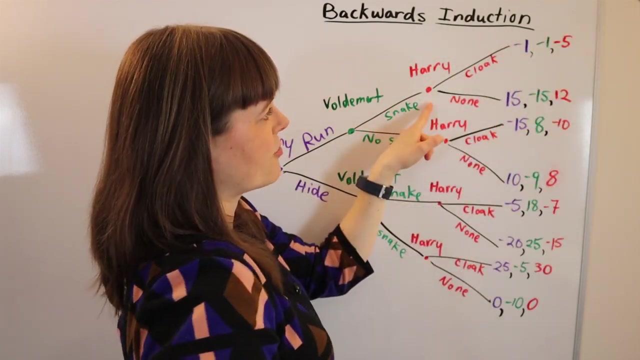 the payoffs they want, and you'll understand that in a second. so what's the process? process of backwards induction is to start at the end of the game, where we we're going to solve every last node first. so this is the last node, since there's no other decisions after it. 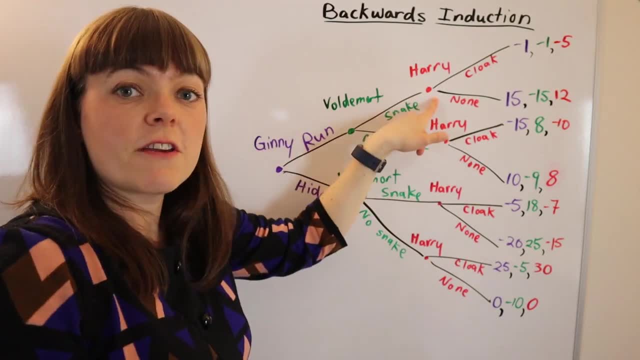 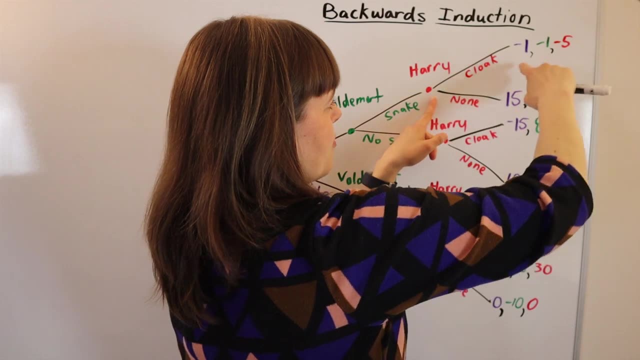 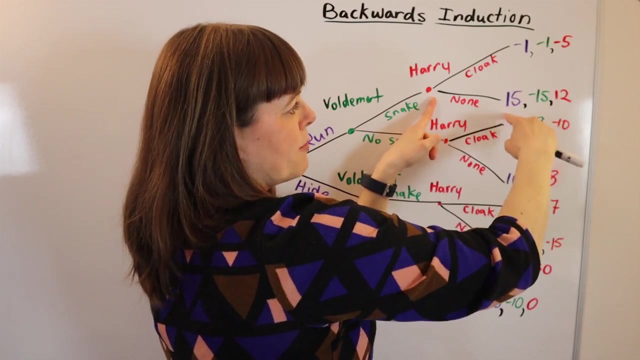 and we're going to look at this node and ask ourselves: if harry finds himself at this node, what decision will he make? and we can see that if he brings the cloak, he gets a payoff of negative five. if he doesn't bring the cloak, he gets a payoff of 12. he prefers the 12.. so if we get to, 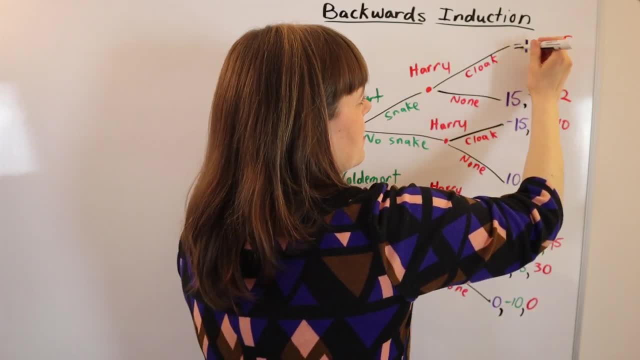 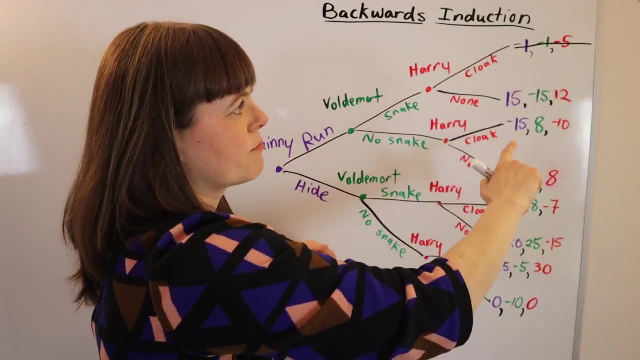 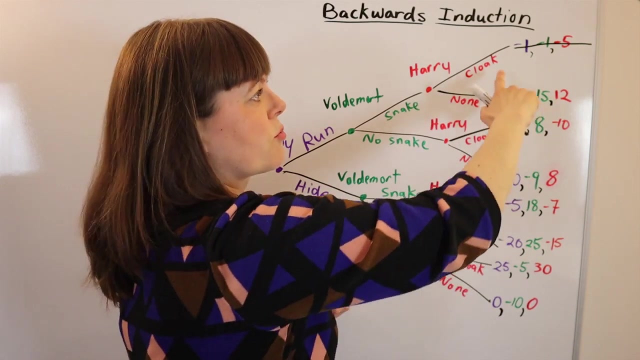 this node. we know we will never reach this, this outcome, so we can actually cross it out so well. actually jenny and voldemort also don't like that, but we know, even if they love, that, even if jenny had a payoff of 100 up here, she would never be able to reach that node, because we know if harry 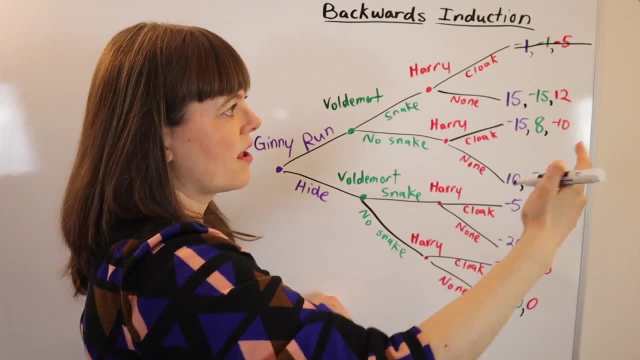 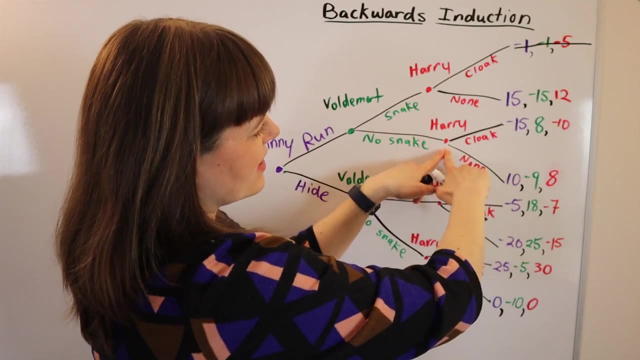 gets to this node, he is not going to bring the cloak. he's going to get a payoff of negative five bring his cloak, and that's the key logic here. so we'll solve every single end node, which, in this case, is all harry's. if harry ends up here, he's going to look at the negative 10, his payoff if 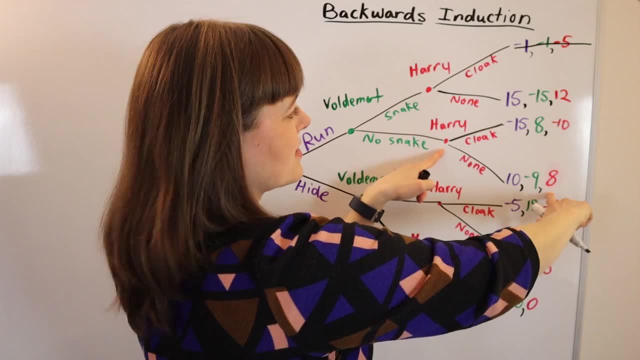 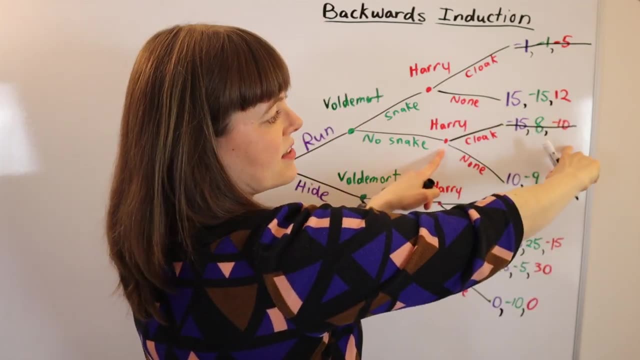 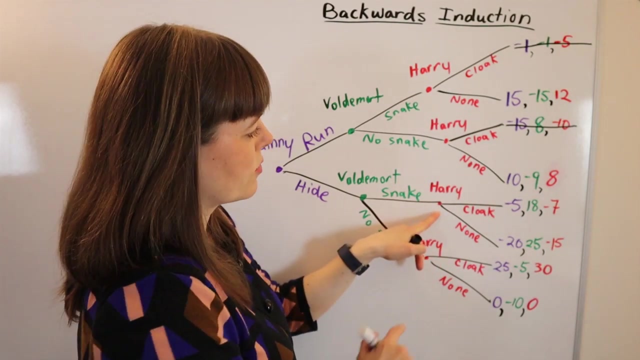 he chooses cloak and he'll look at the eight, his payoff. if he doesn't bring his cloak, he prefers the payoff of eight, so he crosses. so. so everybody is going to cross out that end node as being something that will never be reached. and then we do the same thing for his other two nodes. 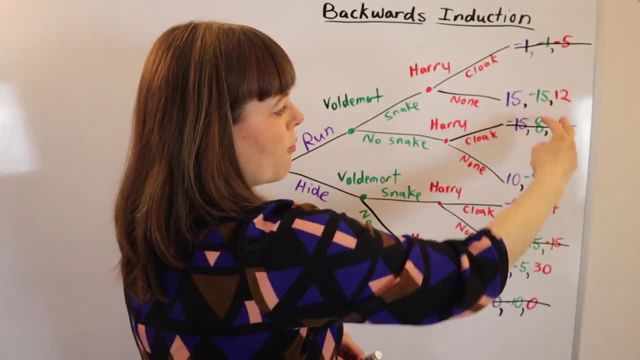 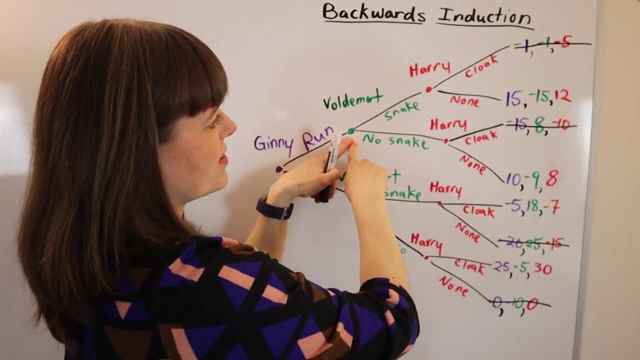 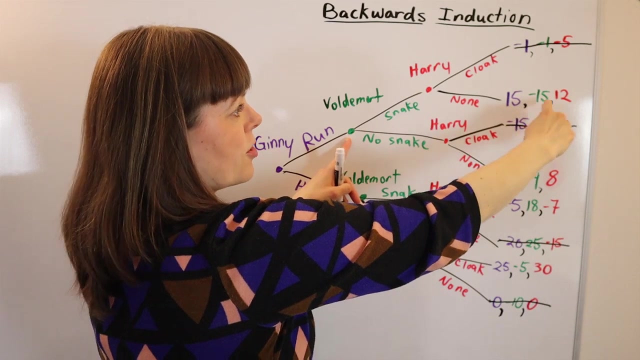 so two other nodes are dead, 4 nodes are still locked and now we have four end nodes left in the game and we can move one step backwards. so we're going to move to voldemort's decision and voldemort is going to say: if i choose to bring my snake, then we're going to end up here for sure. 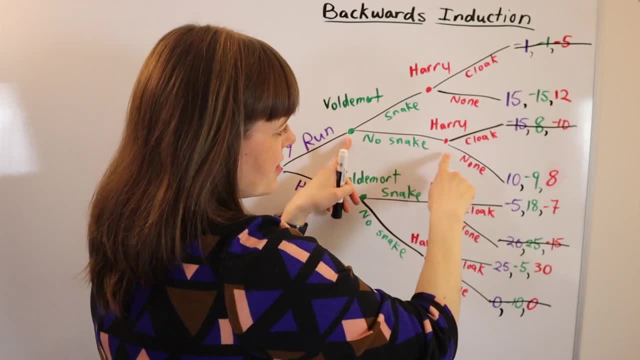 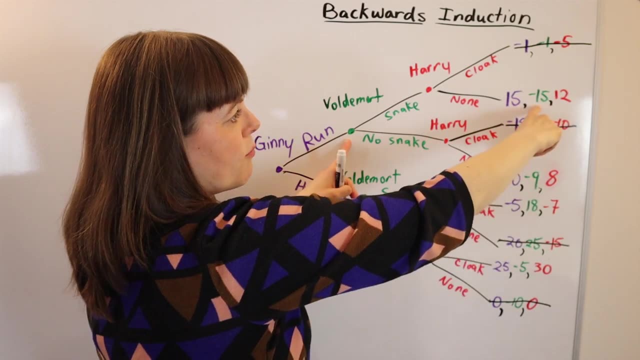 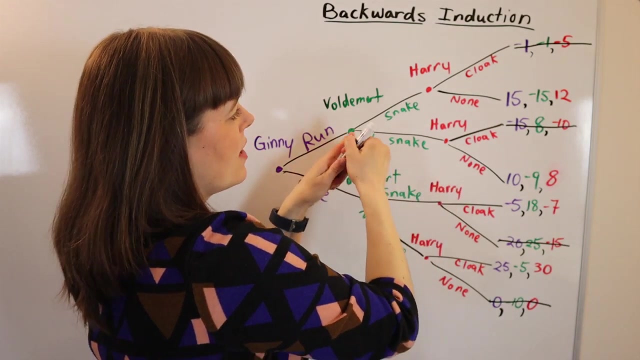 my payoff is negative 15 if i choose not to bring my snake. we know we're going to end up down here and my payoff is negative 9.. he prefers the negative 9 more than in the negative 15.. So he will choose not to bring his snake if he ends up at this node, meaning this node will. 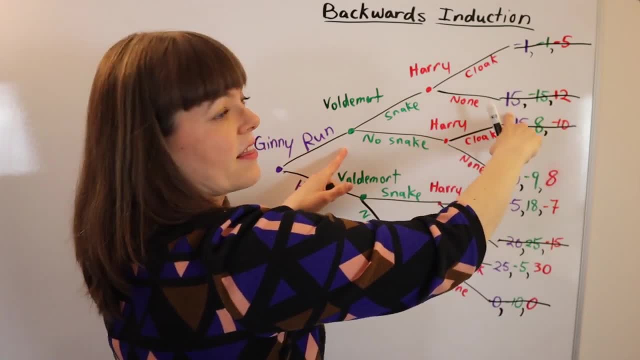 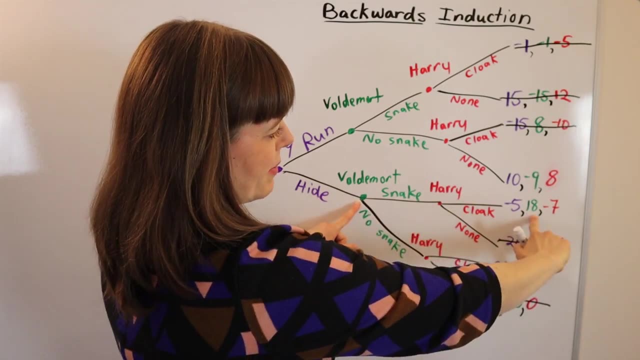 never be reached, regardless of how much Jenny likes that payoff of 15.. And then we do the same thing down here. If Voldemort brings his snake, he knows he'll get a payoff of 18, because we're going to end up here. If he doesn't bring his snake, he knows we're going to end up down here. 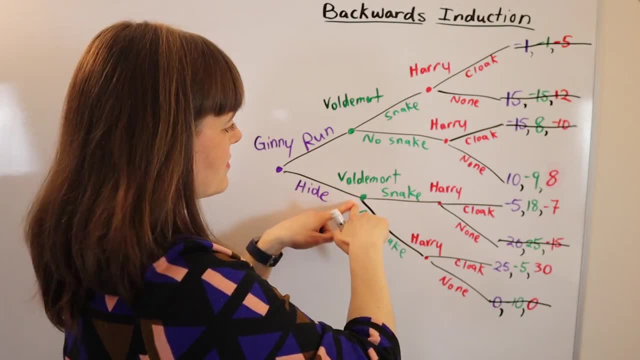 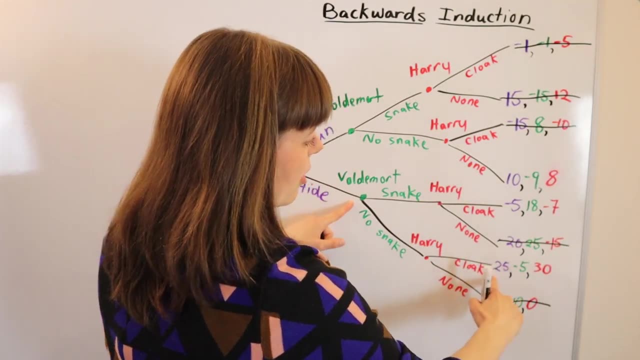 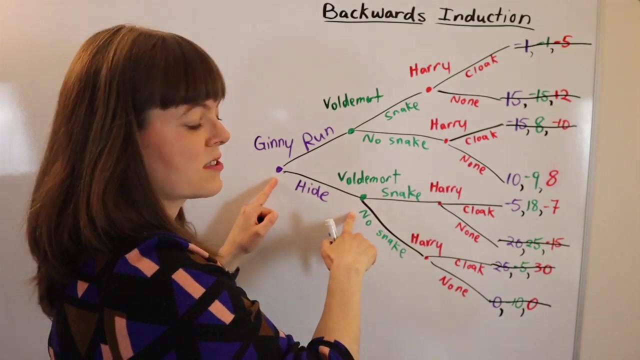 with a payoff of negative five. So if Voldemort finds himself at this node, he will choose to bring his snake, meaning this end node will never be reached. Even though this was actually Jenny's favorite end node, she knows, if she uses backwards induction, that even if she chooses hide. 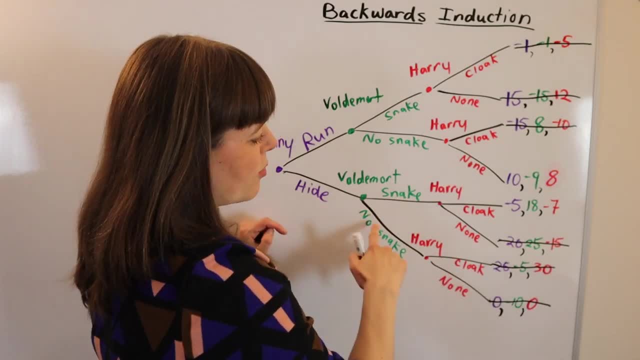 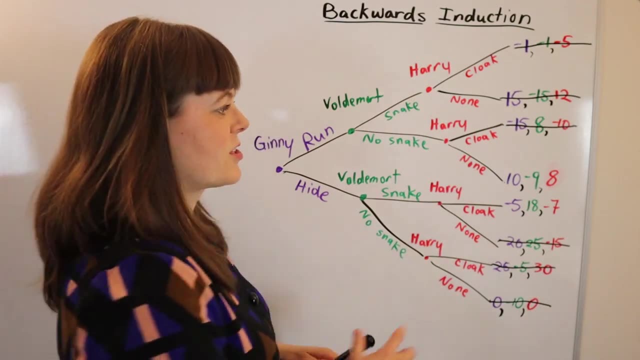 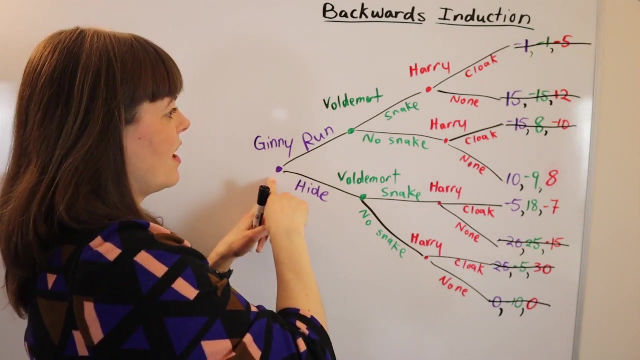 there's never going to be a situation where Voldemort will choose not to bring his snake. Voldemort will bring his snake in response to her hide down here. So now we're left with two possible endings, End nodes, And we move back one step to the beginning of the game, to Jenny's choice, And 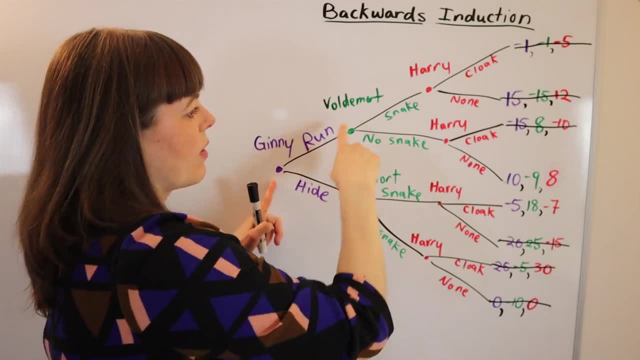 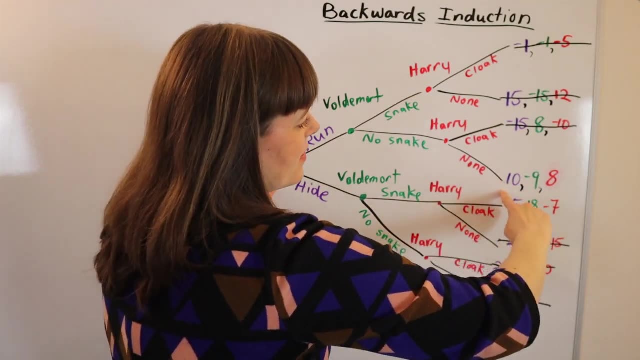 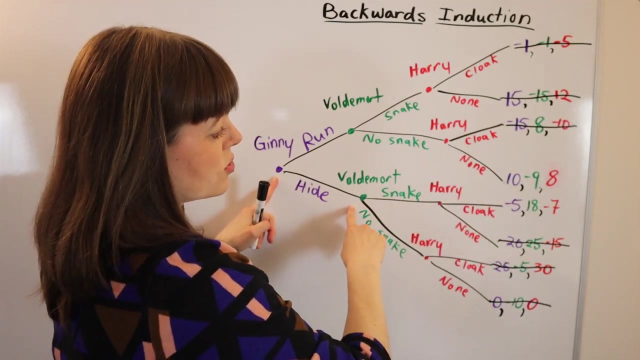 she's deciding: do I run or do I hide? And if she runs, she knows for sure, based on Voldemort's decision and Harry's decision, if they're using backwards induction, that we'll end up over here and she'll get a payoff of 10.. If she chooses to hide, then she knows exactly how things are. 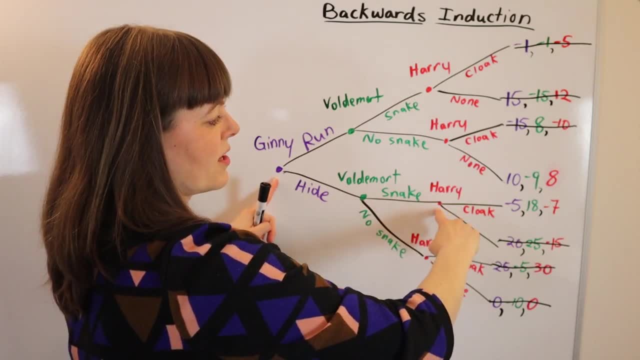 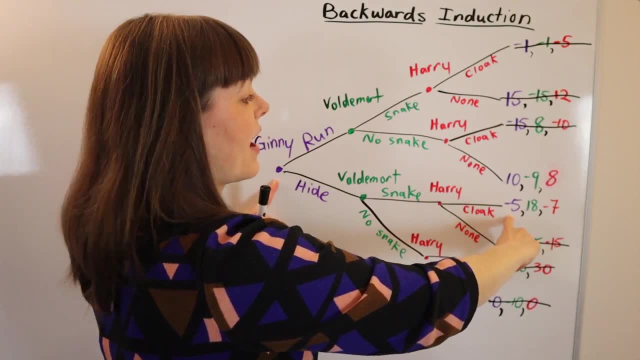 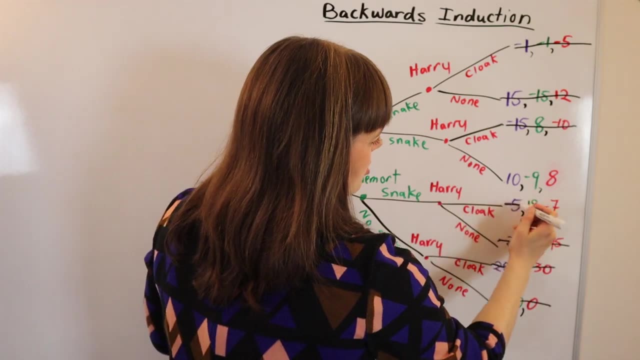 choose to bring his snake, Harry will choose to bring his snake, Harry will choose to bring his cloak, And her payoff will be negative five in that case. So she likes that 10 better than the negative five. So she's not going to choose to hide And therefore the solution to this game is: 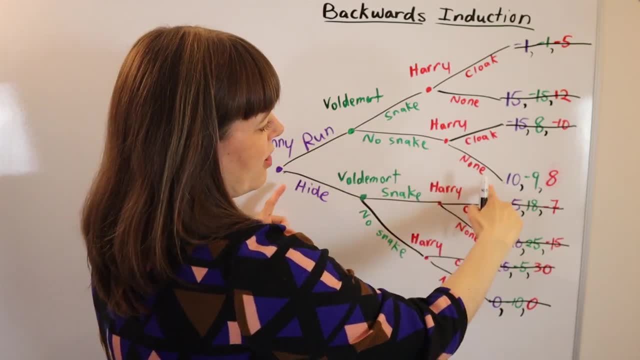 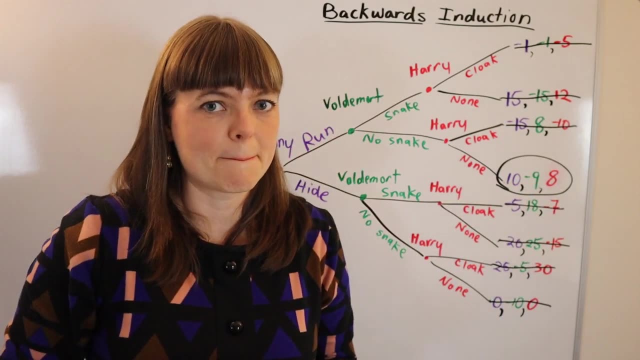 for Jenny to run, Voldemort to not bring his snake and for Harry to not bring his cloak, And this will be the final payoffs for the three players in that game. Let's do one more example. All right, this is going to be an example of capture. 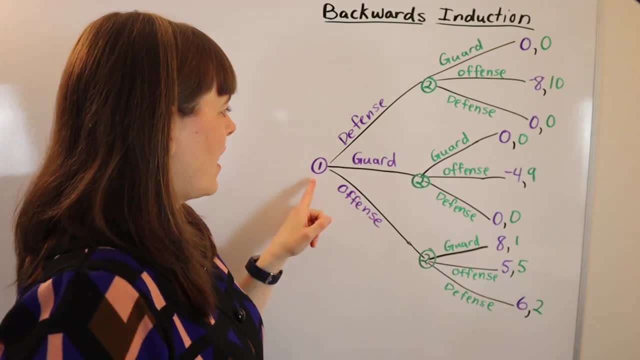 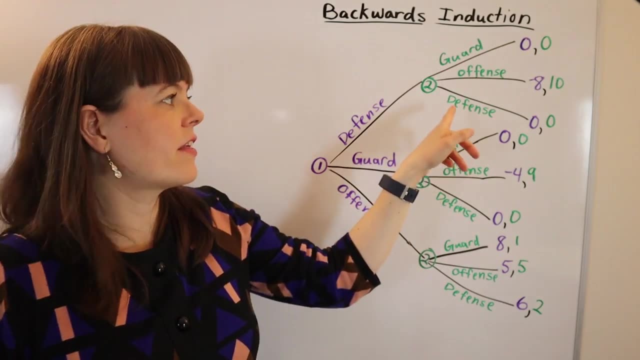 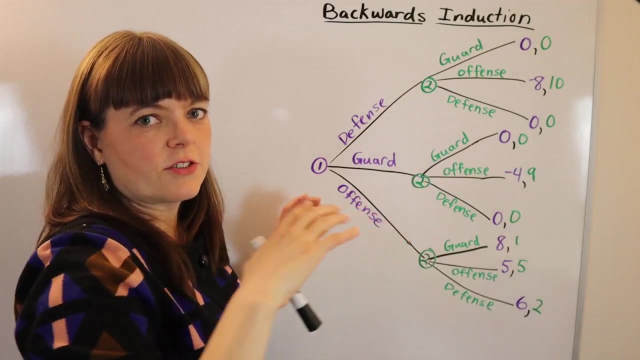 the flag where there are two players left and you're trying to decide what to do, what your move right now should be, given that the other player is going to observe your move and respond. So the three options are: you play defense, you just sort of hold your fort and sort of try to. 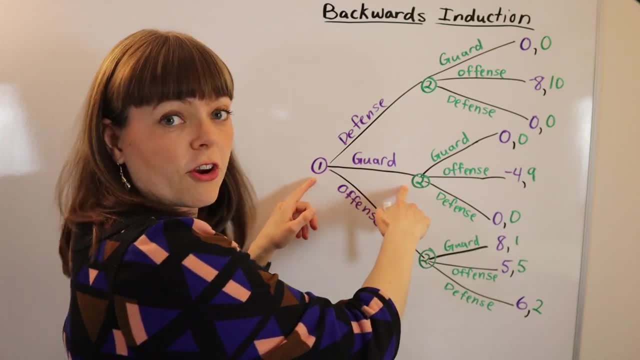 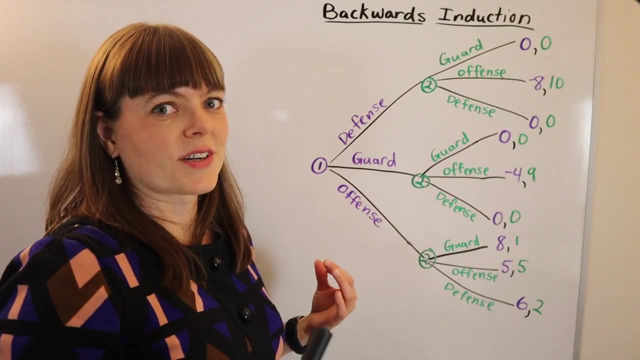 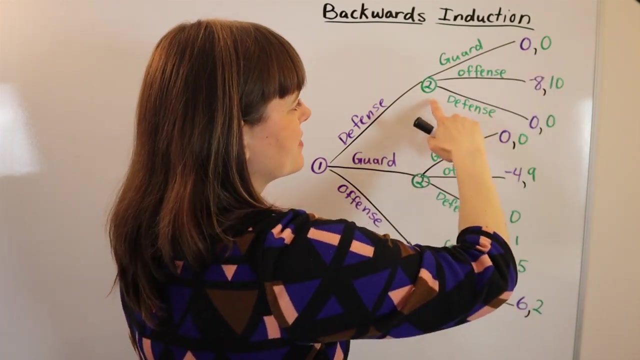 follow them to stop them from coming in. you guard your flag or you play offense, and the other player has the same three options. So, of course, we're going to solve this using backwards induction, by identifying the nodes at the very end of the game that lead to the payoffs and seeing what 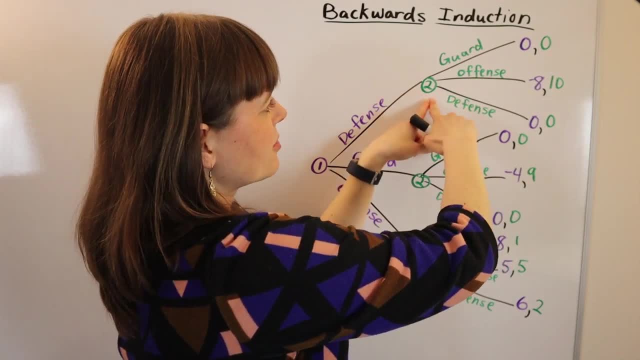 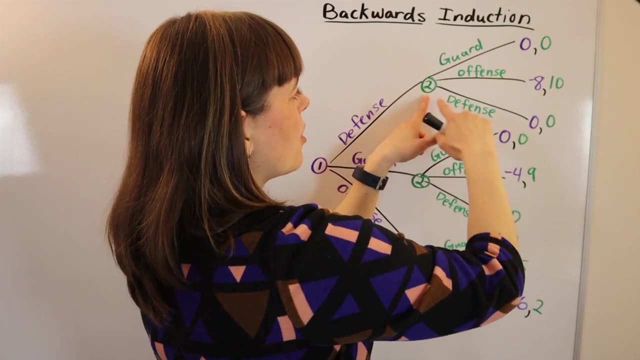 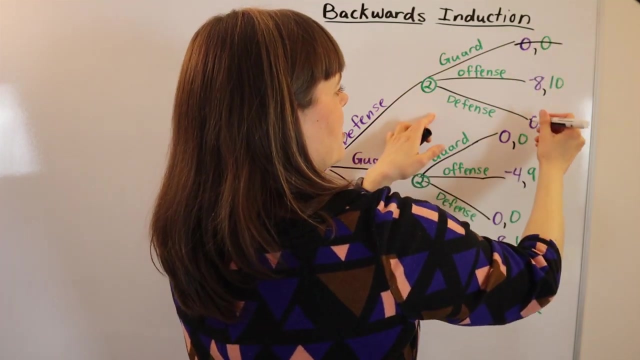 will the player do in each of these cases? So if player two is sitting here, player looks at the possible options and the paths here are going to be zero, ten and zero. So if you choose defense, then player two will definitely choose offense. so we will never reach the end.